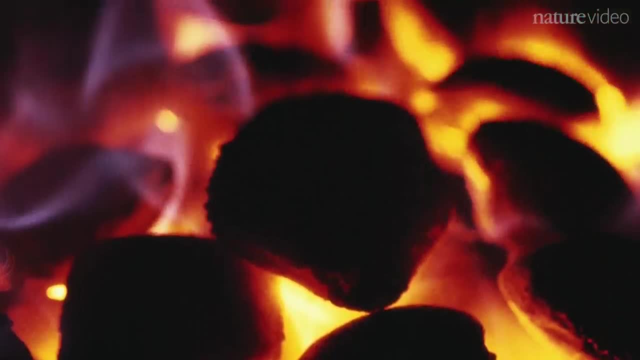 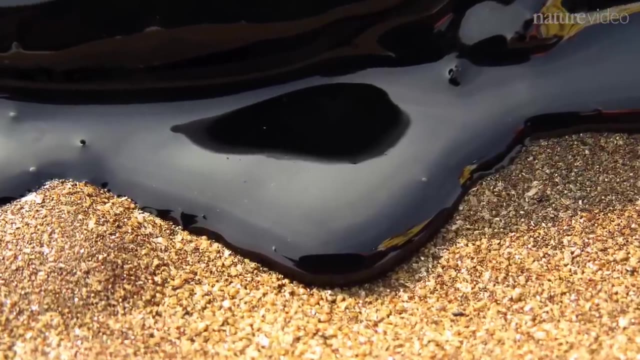 them down as firewood or dig their remains up as coal. But the world's biggest energy source is oil. And can you guess what most of that pressure precious oil is made from? What a surprise It's plankton- Single-celled creatures like. 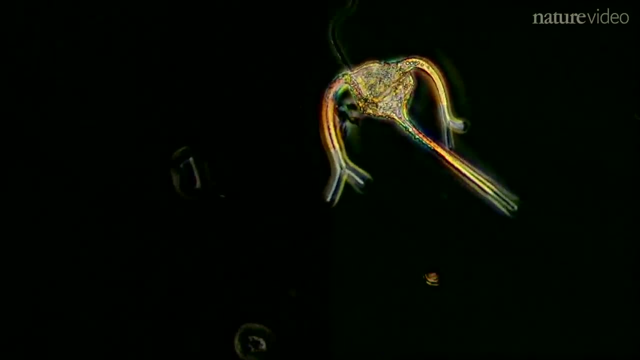 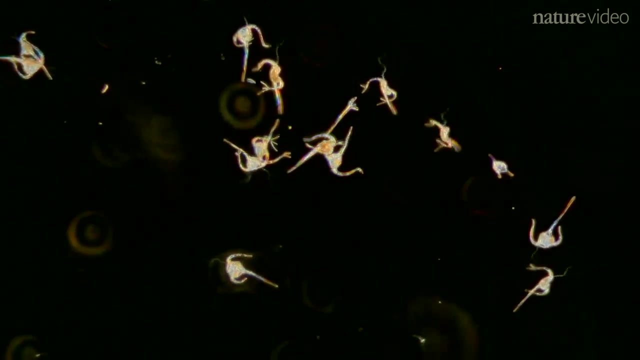 diatoms and dinoflagellates die and sink to the sea floor, where they're crashed and transformed over millions of years into oil and natural gas. Sure, dead trees contribute some of it, But the plankton had a three billion year head start, making them the world's largest. 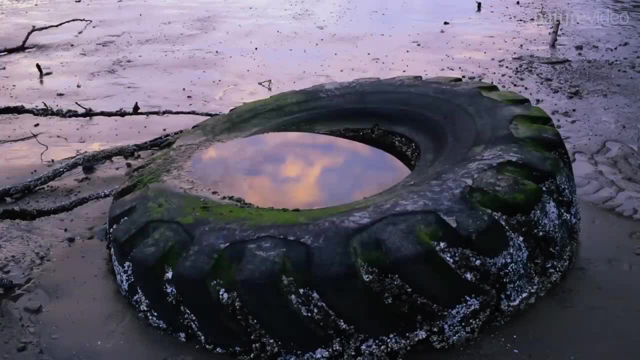 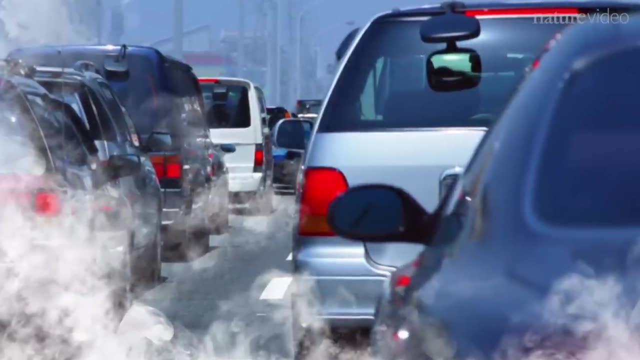 supplier of fossil fuels. So much for saving the planet. Thanks, plankton, Number three rocks. When we're not burning plankton's remains for fuel, we're building houses from them, From St Paul's Cathedral to the Great Pyramids- some of our favourite. 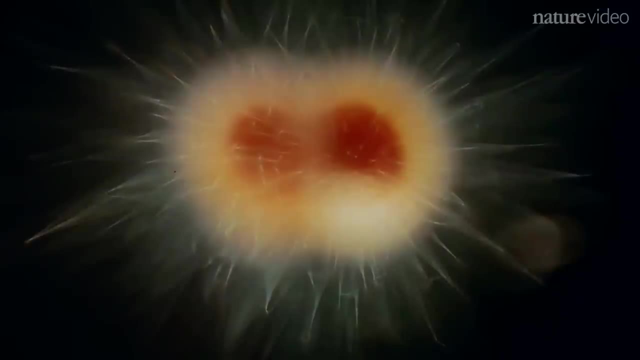 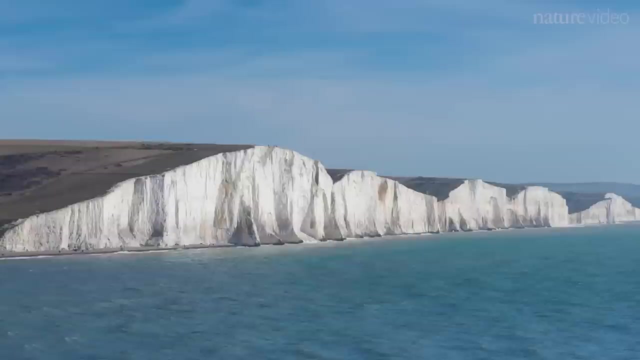 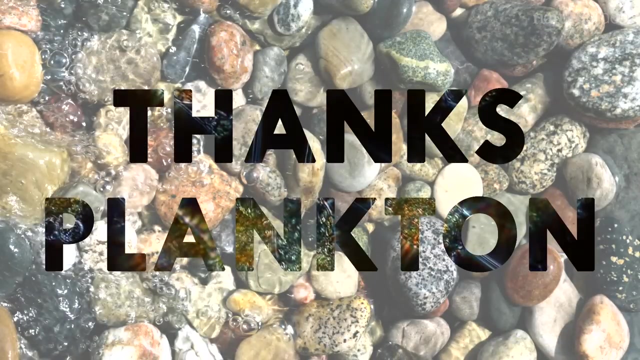 chunks of rock were once at the bottom of the sea. Hard shells like on these foraminifera fall to the ocean floor and end up cemented into sedimentary rocks. Chalk is basically entirely plankton. So what have we learnt? That's right, Plankton rocks. Thanks plankton. 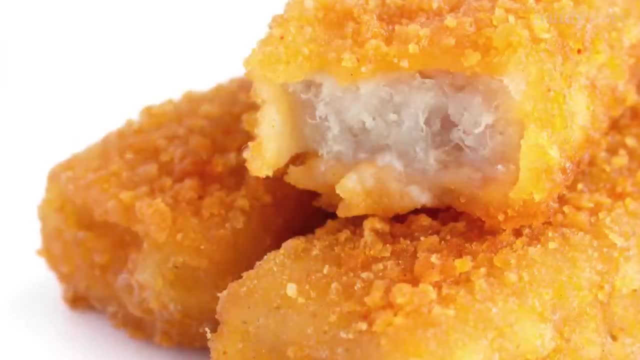 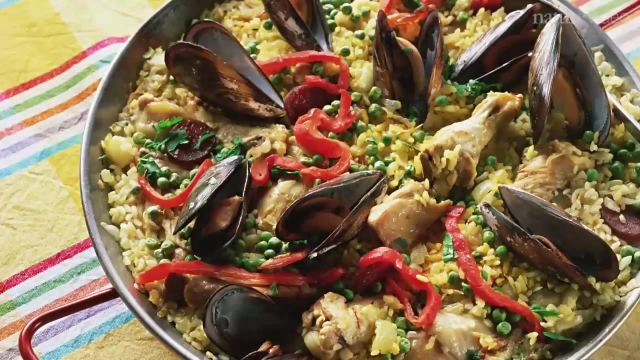 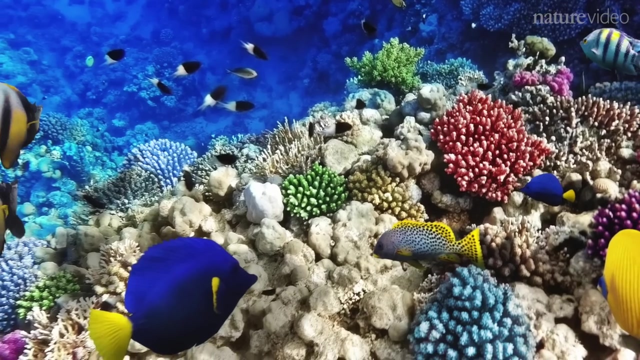 Number four: Fish fingers. Okay, so maybe you can technically survive without fish fingers. Or salmon Sushi, Mussels, Tuna, mayo sandwiches- Okay, let's just say you're vegetarian. The point is, all sea creatures, delicious or otherwise, depend on plankton somewhere. 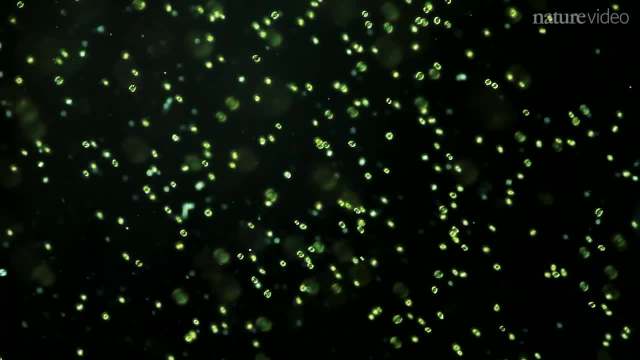 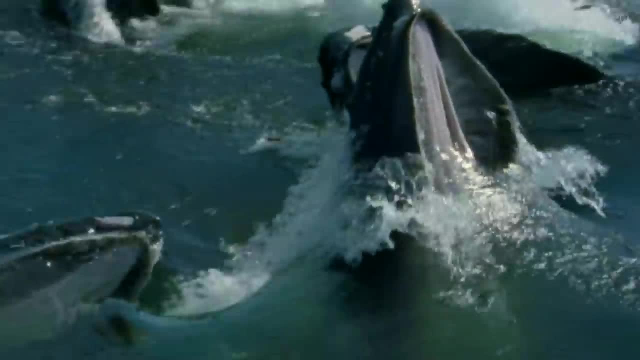 in the food chain. Our pals, the photosynthetic plankton, turn sunlight into food for hungry zooplankton, some of which, like krill, feed ever bigger marine predators. So if you liked Finding Nemo, don't thank Disney, Don't. 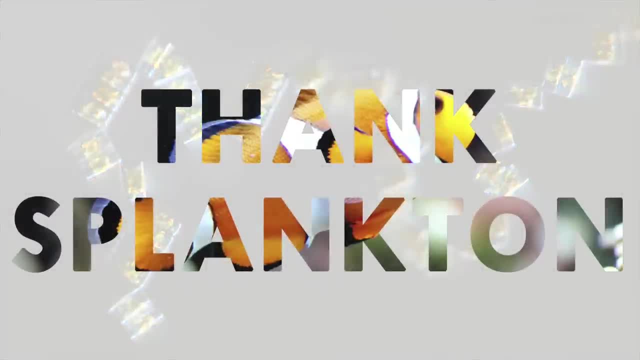 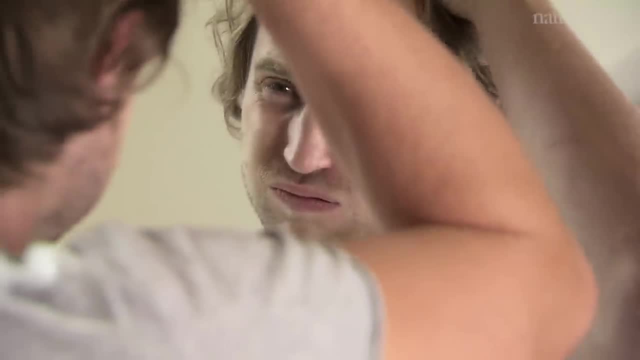 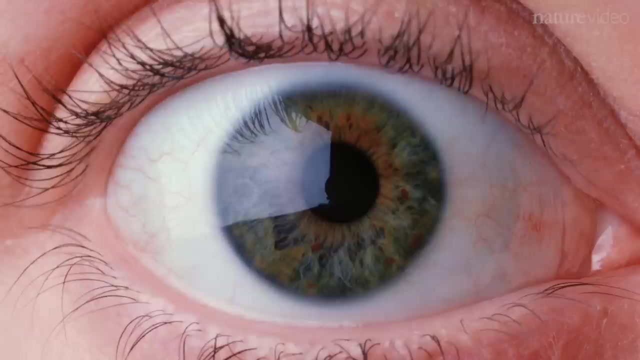 thank Pixar, Thank plankton, Thanks plankton. Number five: Your face. Without plankton, you wouldn't have a face Or legs Or a gallbladder. What I'm getting at here is that we all kind of evolved from plankton.